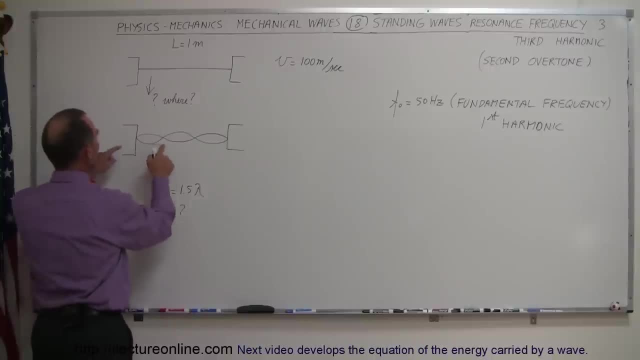 All right. So, First of all, notice that we have two notes at the end, two notes in the middle, for a total of four notes and three antonotes: one, two, three. So what you need to do is you need to plug the string at the location of where you want that antonote to be. 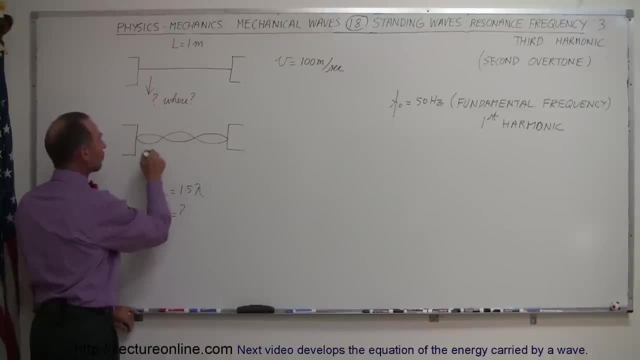 So this is one half of one third the length. so therefore, you want to go to one sixth the length of the string. pull on the string and let it oscillate, And that's what we typically do with guitar strings or violin strings. 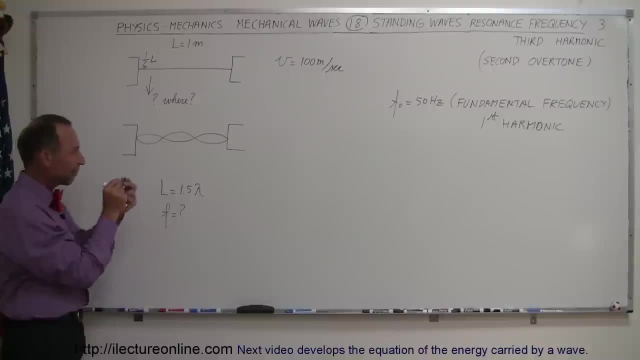 We stroke Or we strum Or we pluck the string at a particular location to set a particular waveform like that, Whatever it is that you're trying to obtain. So if you pluck it one sixth the length of the string, you'll end up with a pattern like this: 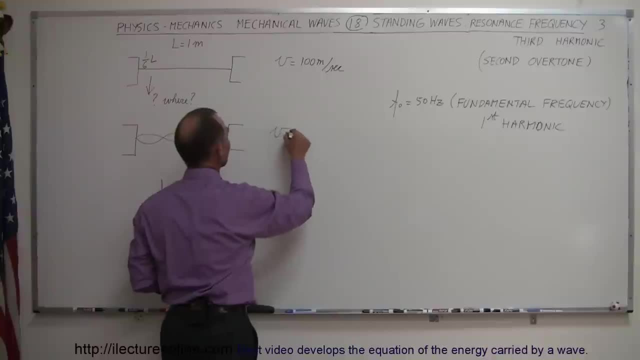 So what is the frequency? Well again, velocity is equal to frequency times wavelength, which means that the frequency is equal to the velocity divided by the wavelength And, of course, the velocity stays the same: at 100 meters per second. It's the wavelength that keeps changing. 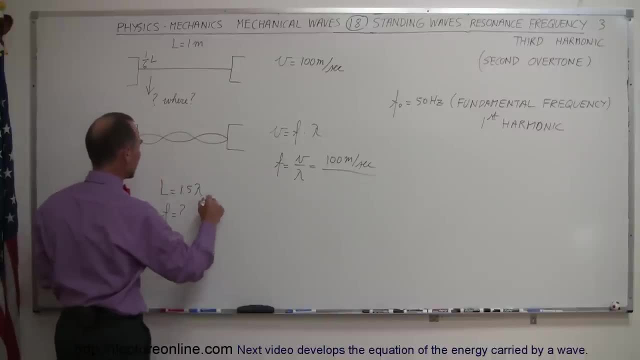 Now notice the length: It's one half lambda, which means from this we can then conclude that lambda is equal to L divided by 1.5, which is 1 meter, divided by 1.5, which is equal to 0.67 meters. 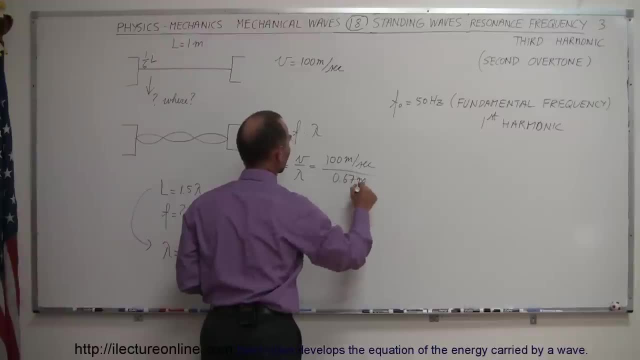 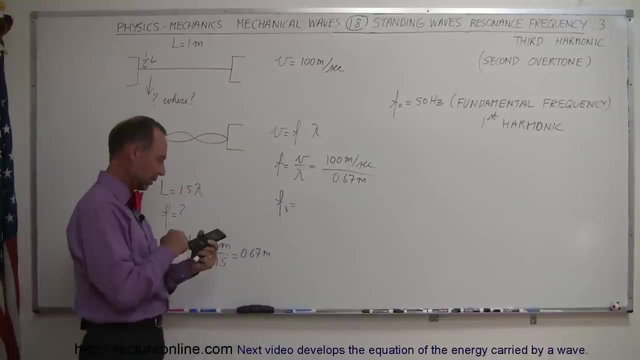 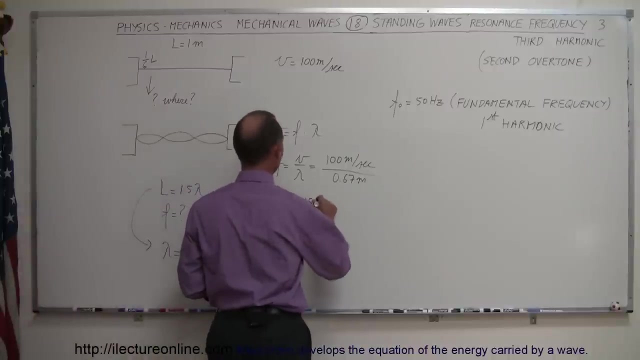 And that goes in here. 0.67 meters. Meters cancels out. And the frequency of the third harmonic, 100 divided by 0.67, is Wow- Good thing I checked. That's equal to 150 hertz. 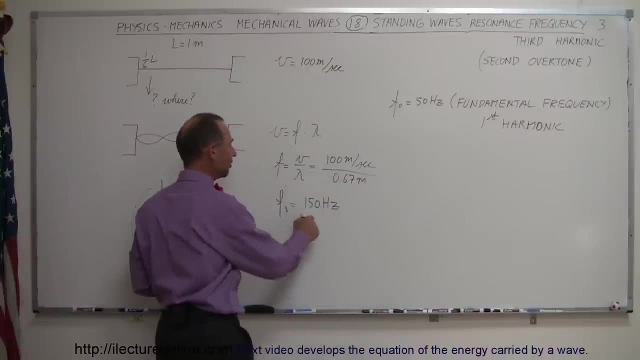 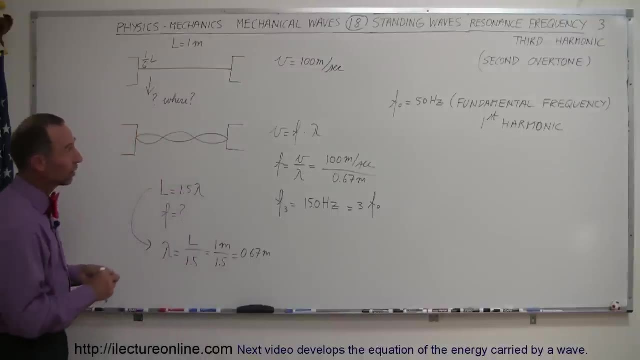 And now that I think about it, yeah, that should be the answer, Because this is three times the fundamental frequency. So notice that with the second harmonic the frequency was 100 hertz, which is twice the fundamental frequency, And with the third harmonic that is now, as we see, three times the fundamental frequency. 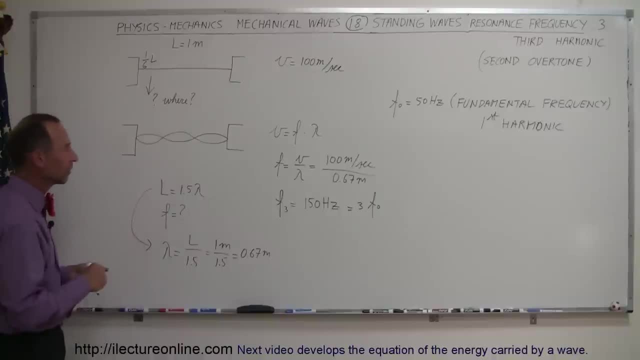 So, for each harmonic, it's simply a multiple of the fundamental frequency, And that's how we find out what this is. So, now that we have the pattern, if I asked you what is the frequency of the fifth harmonic If we have five of these, five of these lobes, or five of these half waves oscillating up and down?